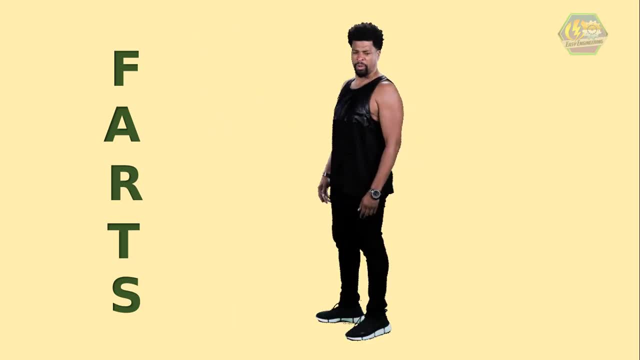 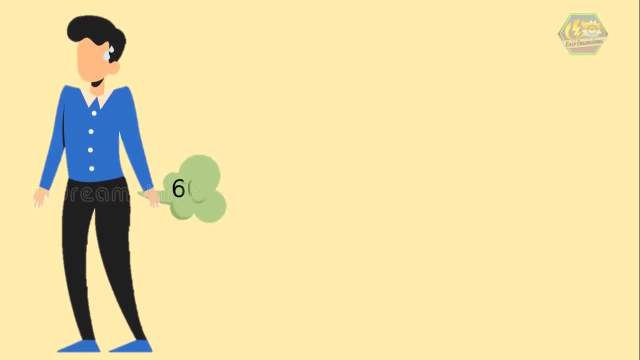 They're stinky and they make a funny sound, But the thing is, our farts contain a very important particle called nitrogen. In fact, there's about 60% of nitrogen inside them. Nitrogen is very essential to how we live. 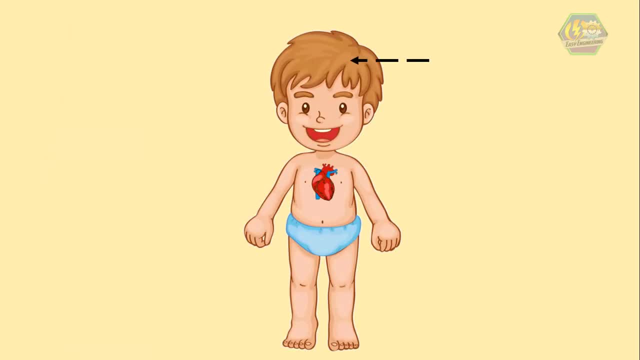 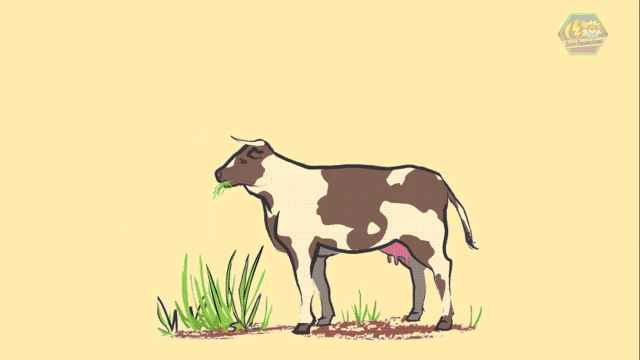 It can be found in everything from your hair to your organs. The air we breathe contains a lot of it. Now, some of us might want to ask: why is nitrogen important to life? Plants and animals could not live without nitrogen because it is an important part of cells and processes in their bodies, like amino acids, proteins and even our DNA or our genetic code. 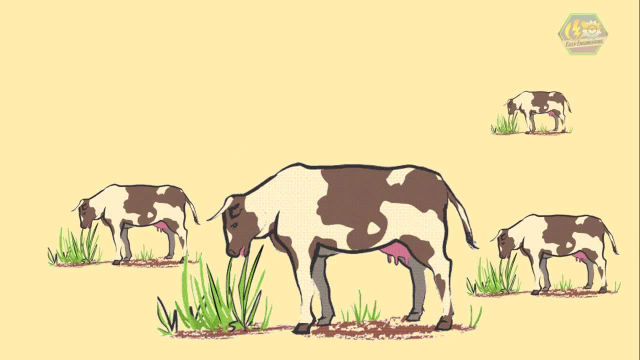 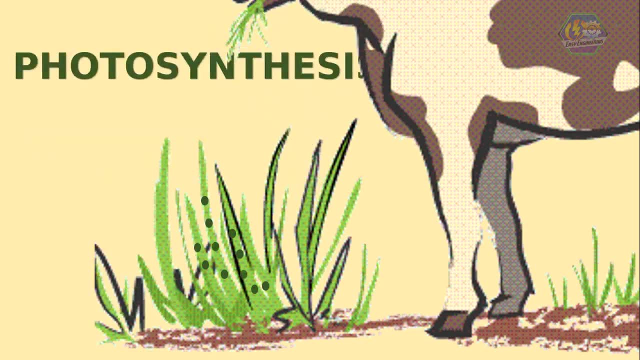 Without nitrogen we cannot replicate or produce another living thing. It is also important in plants to make chlorophyll. This substance is used in photosynthesis to make their food and energy. But plants and animals don't absorb nitrogen that easily, Even if there's a lot in the air. we all need another way to obtain the nitrogen. 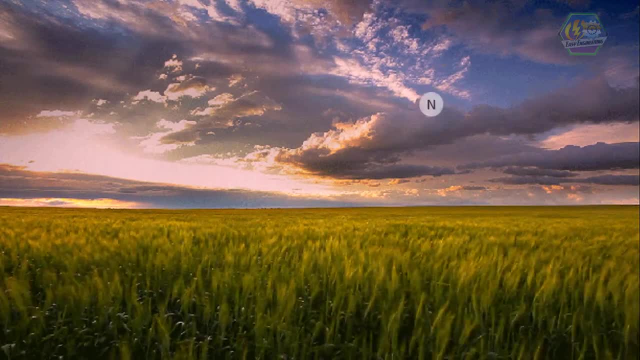 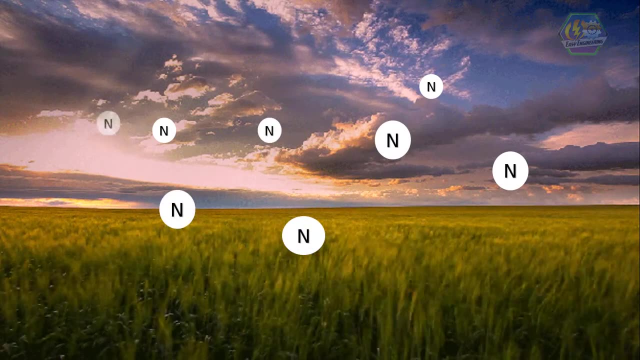 Nature has a way to automatically provide us with nitrogen, and it involves processes to get nitrogen out of the air and into living organisms. This is called the nitrogen cycle. What is it and how it is important to us. Let's dive in and find out. 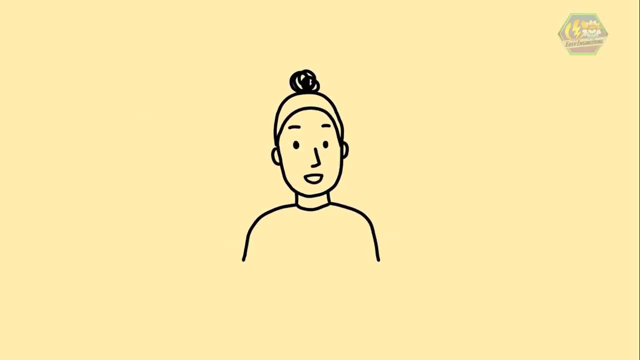 Fun fact learners. did you know that the air you breathe from the atmosphere is? the air you breathe from the atmosphere Is about 78% nitrogen. Well, yes, that's almost all of the air. For nitrogen to be used by living things, it needs to change into different states. 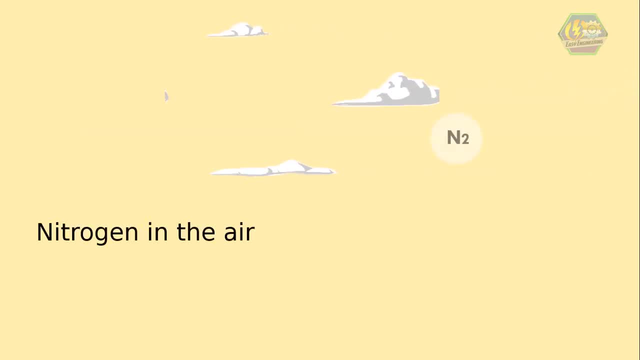 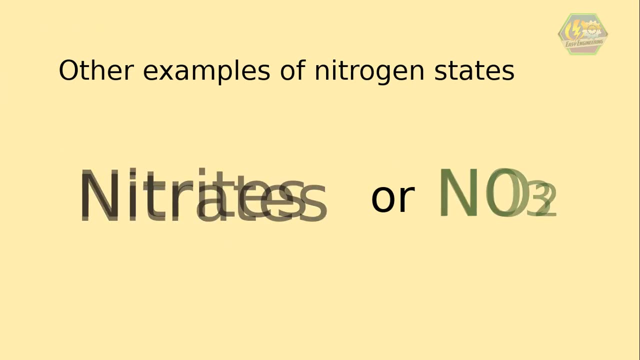 Nitrogen in the air is called N-2.. Other examples of nitrogen states are nitrates, nitrites and ammonium. Fun fact learners: did you know that the air you breathe from the atmosphere is the air you breathe from the atmosphere? 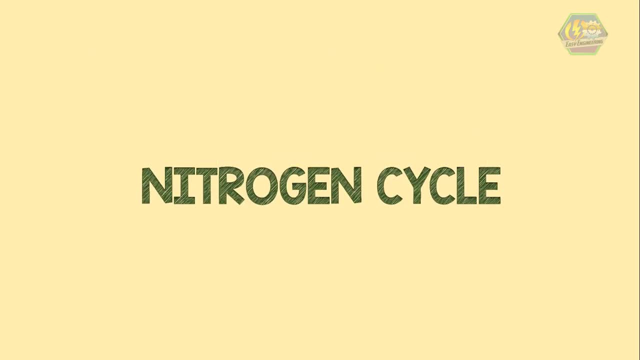 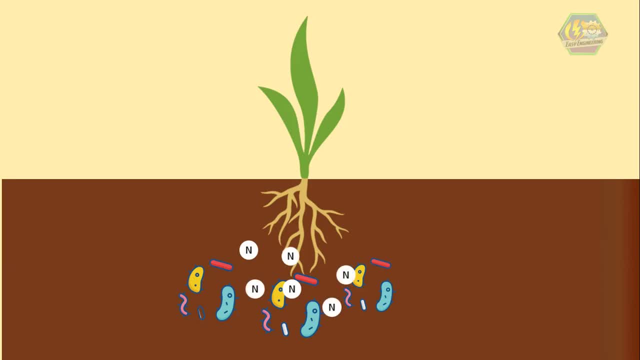 Fun fact learners. did you know that the air you breathe from the atmosphere is the air you breathe from the atmosphere? help it to change state so it can be absorbed by plants, and so we and other animals get nitrogen from plants. the processes involved in the nitrogen cycle. 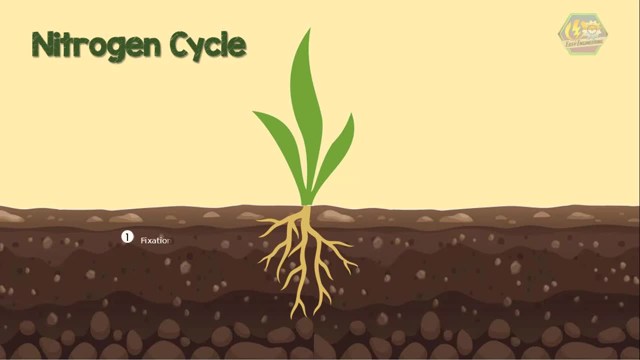 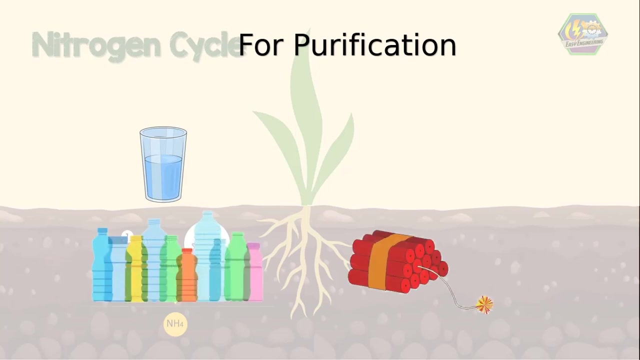 are the following. first is the fixation. it's the first step, for bacteria change nitrogen into ammonium. it's a very smelly kind of gas for us humans. we use ammonium for purification of water supplies and in the manufacture of plastics, explosives, textiles, pesticides, dyes and other chemicals. the second step: 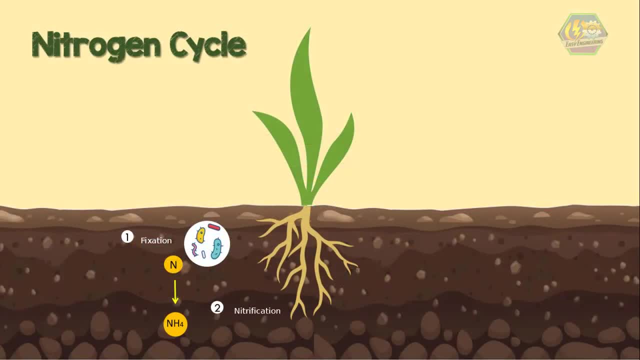 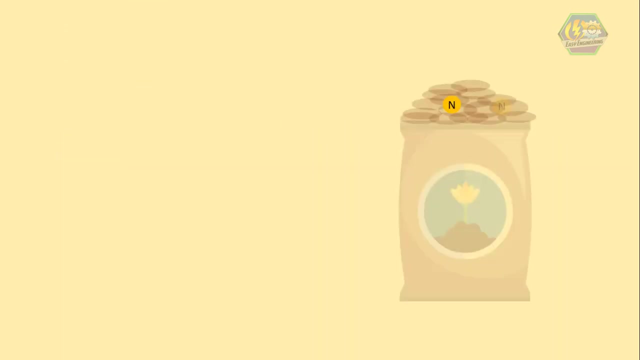 in the cycle is nitrification, like its name. this is where ammonium gets changed into nitrates by soil bacteria. plants can now absorb nitrogen in the form of nitrate. fun fact learners. speaking of absorption, did you know that nitrogen is grown faster? yes, indeed, agricultural engineers are always developing some.